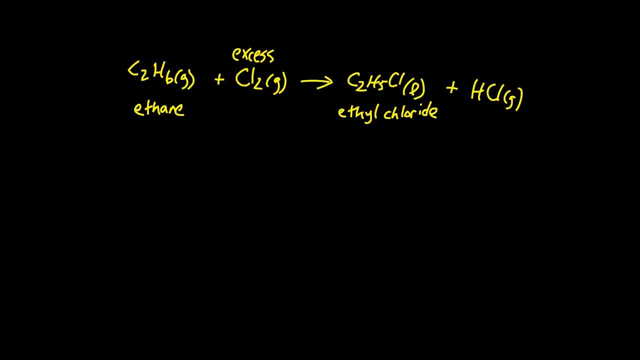 And you know that there's actually a five point: 4.5 grams of ethyl chloride produced and 4.7 grams of ethane put into the reaction. And they want to know is, or what they want to know is, rather, is what's the percent yield? 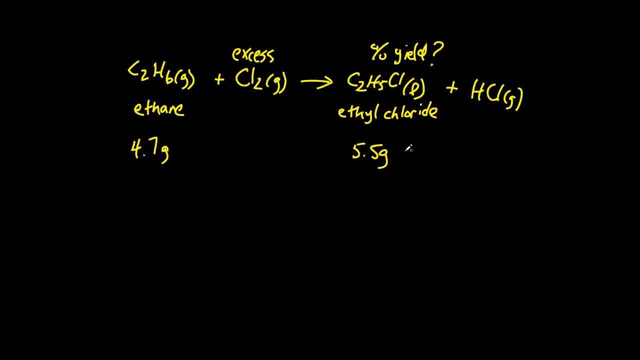 Of the ethyl chloride. That should tell you right away that, if this 5.5 grams is given, this is what they actually got, Which could have been more or could have been less than the theoretical yield, since percent yield is actual over theoretical. 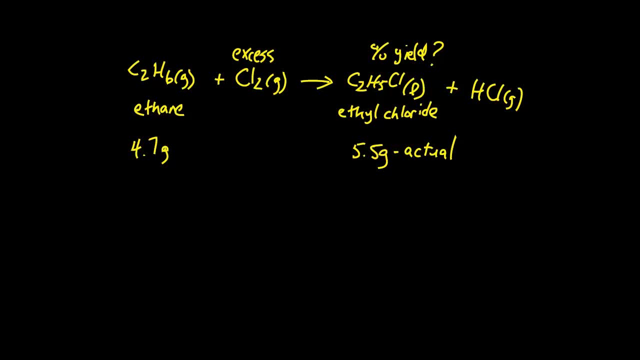 So let's break down the problem into: 1. A mass molar mass mole table. So we have mass molar mass and mole And mass molar mass mole. I'm not going to be concerned with this chlorine since it's in excess. 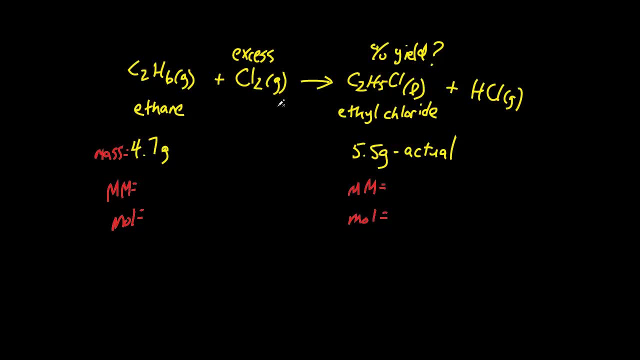 And since that would imply that ethane is our limiting reagent, that means all of the ethane is reagent To get all of the ethyl chloride that we have, And this HCl is not important because it really doesn't determine how much ethyl chloride. 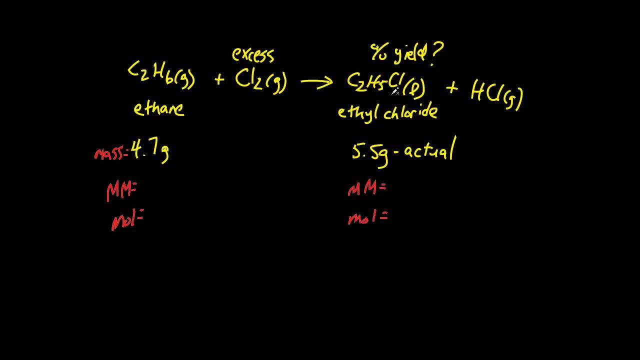 we're going to get. So since the focus of this reaction is just the ethane and the ethyl chloride, I'm only going to bother making my mass molar, mass mole tables for these two guys. And so let's complete. 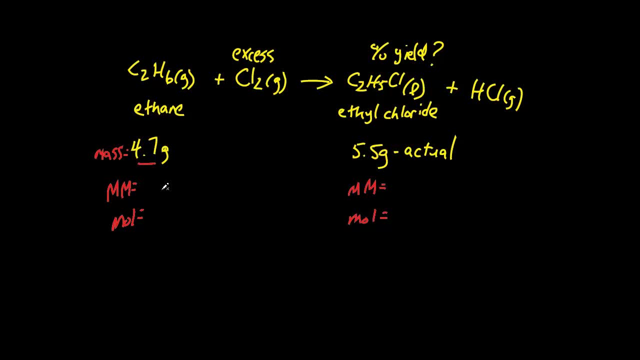 We have 4.7 grams of ethane And we know from the periodic table that the molar mass of ethane, well, it would be 2 carbons, which is 12,, that's 24 plus 6,, that's around 30 grams per mole. 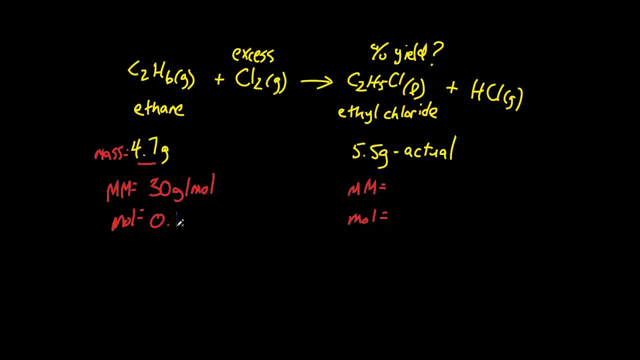 And since we know that moles mass over molar mass, this is about 0.14 mole, So we're going to take that. And since we know that moles mass over molar mass, this is about 0.14 mole. 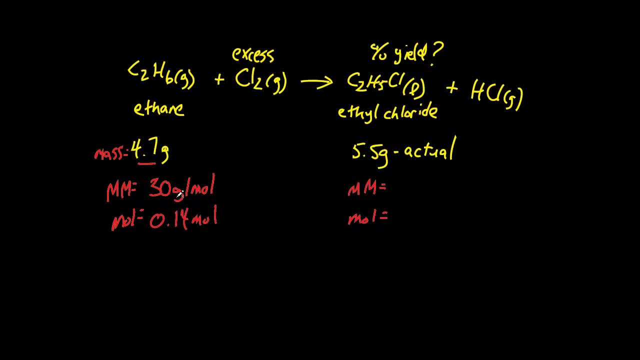 And since we know that moles mass over molar mass, this is about 0.14 mole. Now remember, if we shift our attention now to the ethyl chloride, the 5.5 grams was the actual. Okay, theoretically we should be getting something else. 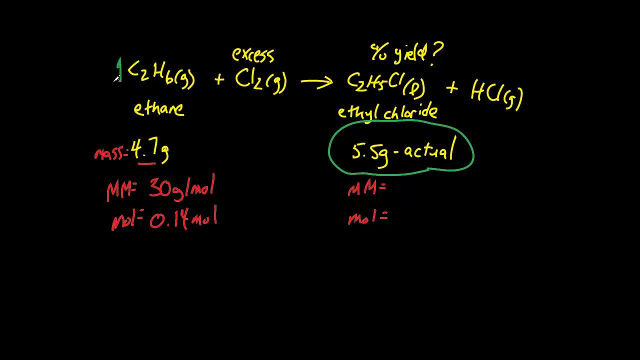 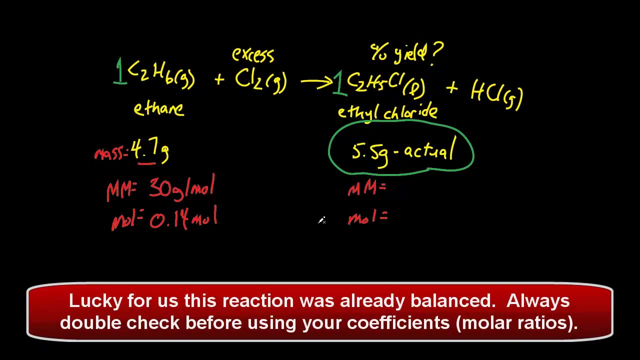 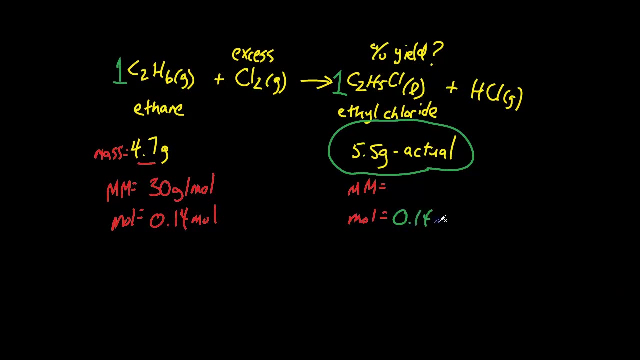 How can we figure that out? Well, if we know that there's a 1 to 1 molar ratio of ethane to ethyl chloride, we can then determine that if we have .14 moles of ethane going in, we should get .14 moles. 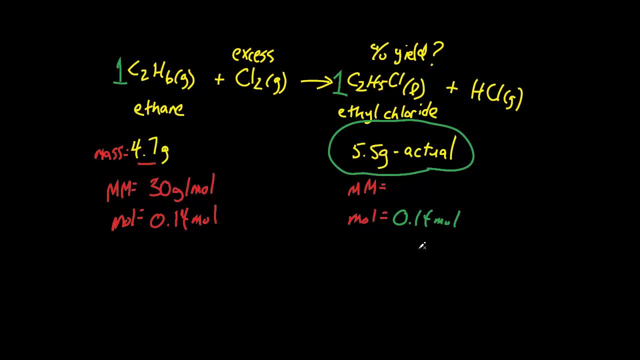 of alpha chloride coming out. Remember, that's what we should get. That's not what we actually got, So don't get those two confused. If we know from the periodic table that the molar mass of alpha chloride is 65 grams per, 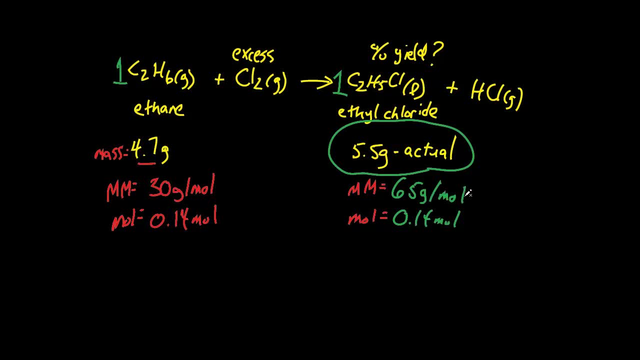 mole, because you have two carbons, five hydrogens and one chlorine, which is about 36, then that means we could easily determine the theoretical yield of ethyl chloride, which is just mass. 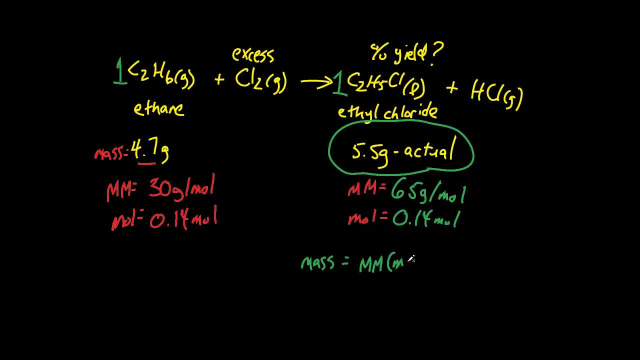 equals molar mass times mole, And if we combine the 65 grams per mole with the 0.14 mole, well, what we're going to get is around 9.1 gram of ethyl chloride. This is our theoretical mass. 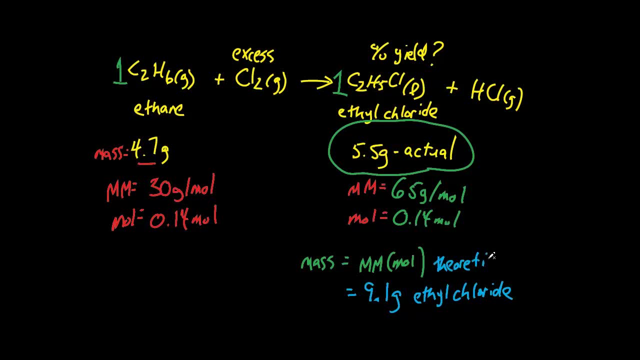 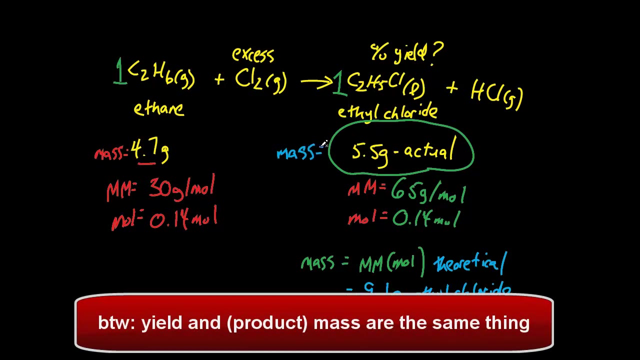 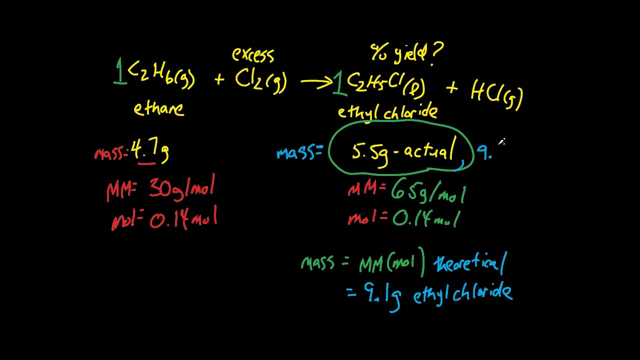 Okay, Okay, Because in theory that's how much we should get. So I'll write this over here: That our mass for this guy is actually 5.5 grams actual- and I'll put a comma there- and 9.1 grams theoretical.